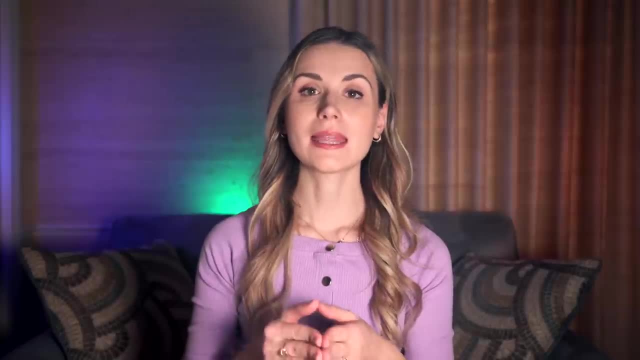 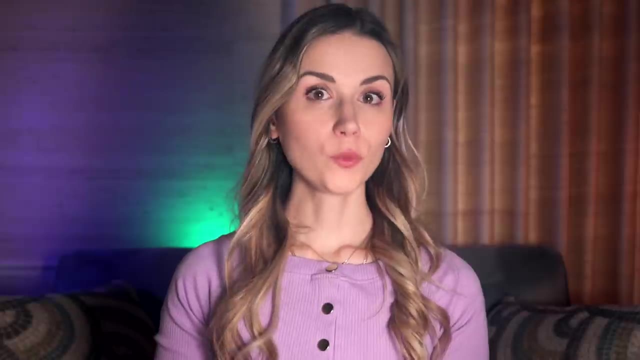 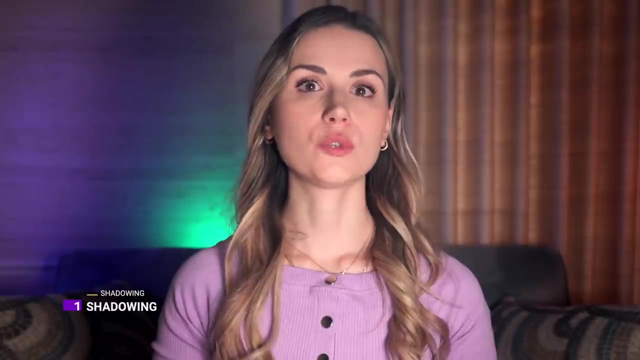 effective exercises to work on your speaking, And then I'll tell you about that one best way to improve your speaking skills. So let's get started. 1. My number one go-to exercise that I recommend to everyone is shadowing. If you really make yourself do it regularly, I promise you will see amazing results. 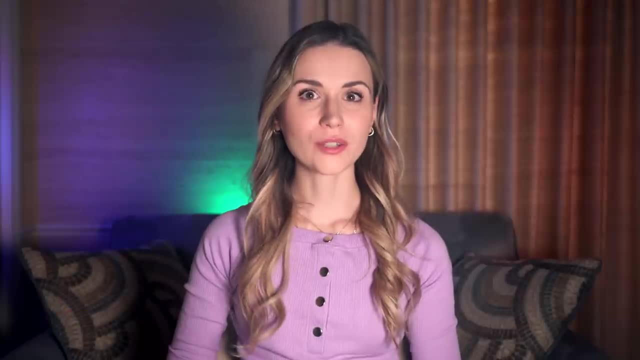 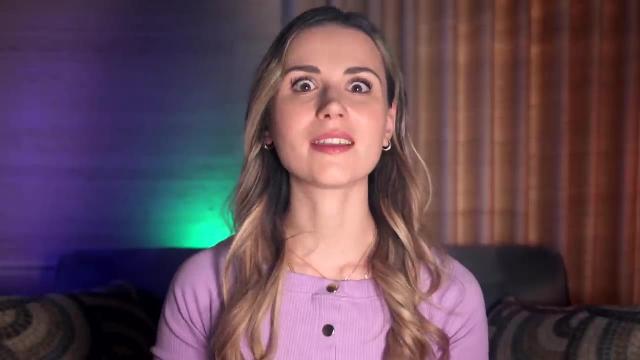 This exercise works wonders. If you want to learn more about it, you can click the links in the description to watch the videos where I talk about it. Next, I recommend that you practice your speaking using my dialogue videos: Little self-advertisement Based on the feedback that I've. 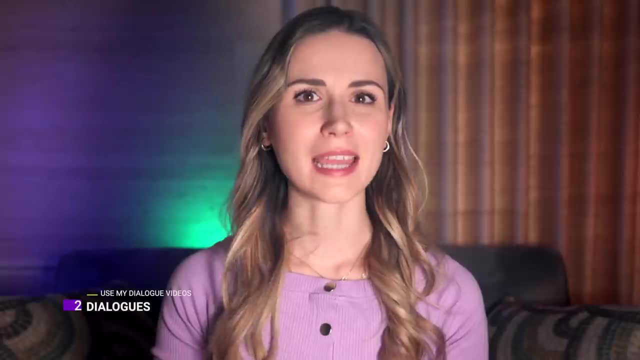 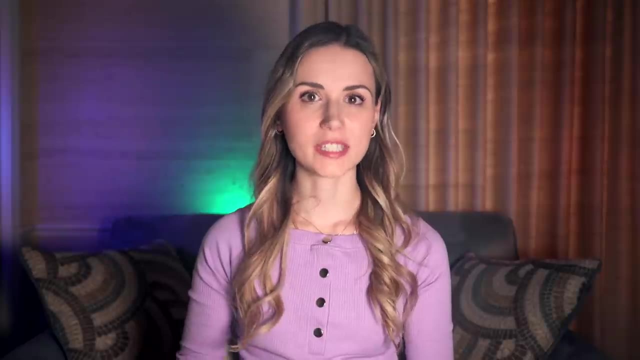 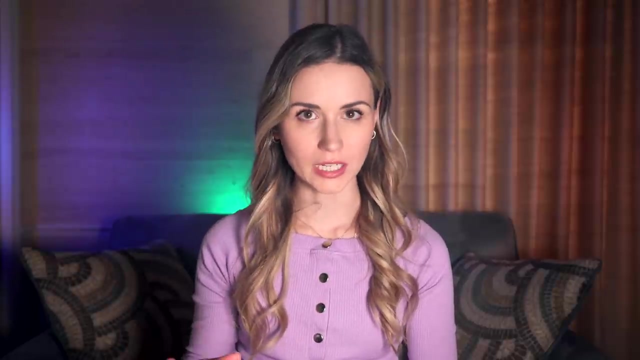 got from you guys on those videos. I can proudly say that this method has helped a lot of you to improve your speaking. In those videos. we basically have a conversation where you and I have our lines and I say my line and then you will see your line on the screen and you need to. 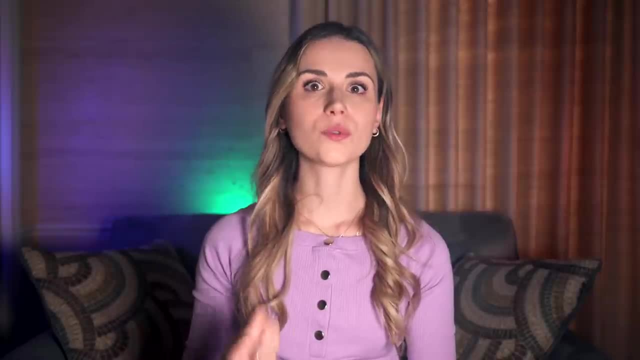 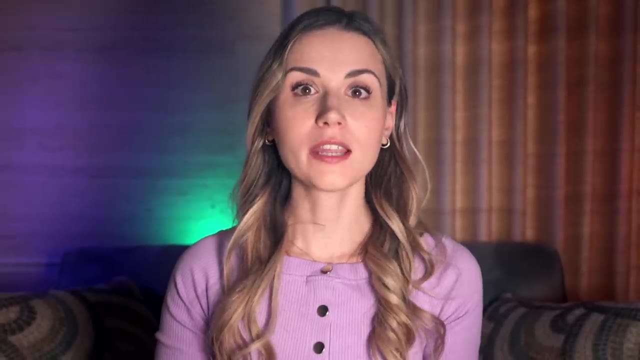 read it out loud off of the screen, as if you were answering me, And I also perform the full dialogue for you. It's easy and fun. 2. Another way is to find dialogues online and read them out loud. Oh, and before I forget to mention this, 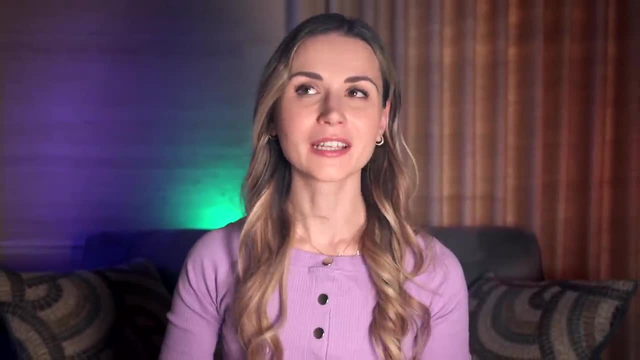 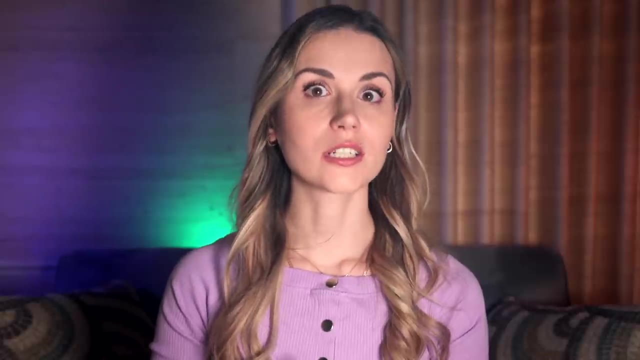 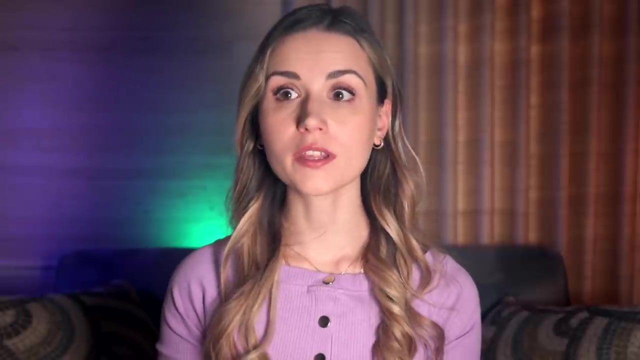 you need to speak out loud. I hope it's clear, because there's no chance of improving your speaking if you don't speak. These two exercises that I just suggested are easy but so effective. Easy because you don't need to come up with your own sentences. You have everything, all. 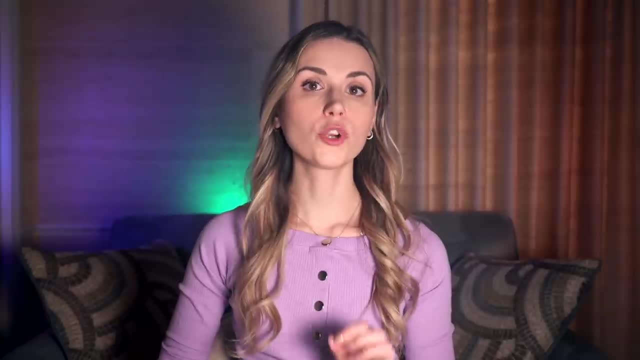 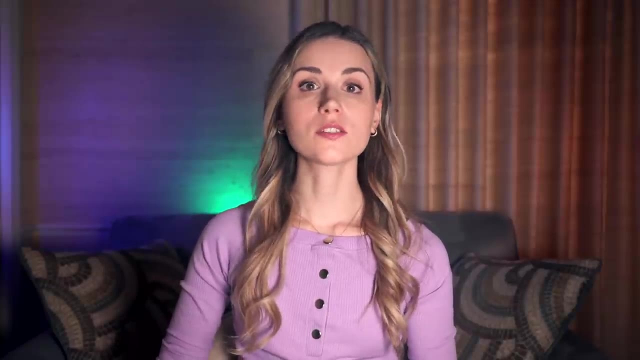 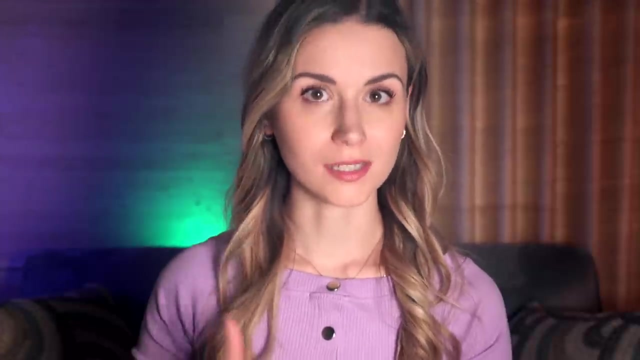 said and done and ready for use. Effective, because the more you actively use the language, the better and easier you learn and memorize things, including grammar, sentence structure, patterns, vocabulary. everything just falls into places On one condition, of course: consistency. 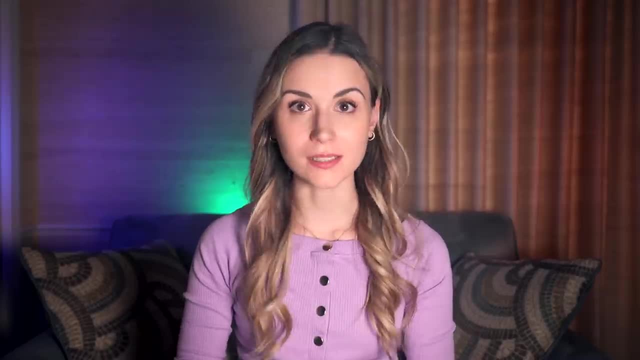 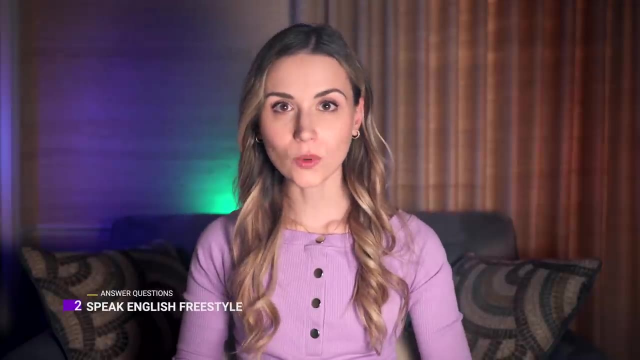 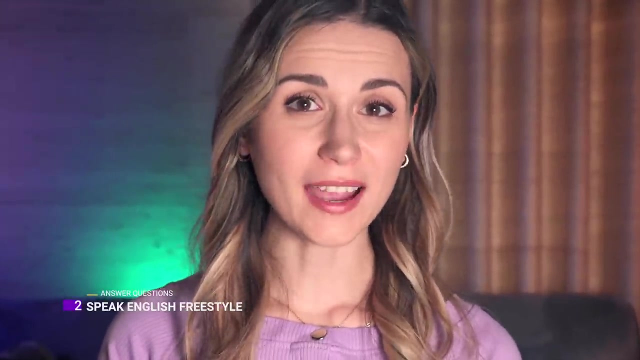 And one more exercise that will help you tremendously not only improve your speaking skills, but also learn to think in English- is to answer questions or speak on some topic in English freestyle Answer whose questions you might ask. well, Google's Search for IELTS speaking test questions or small talk questions, which 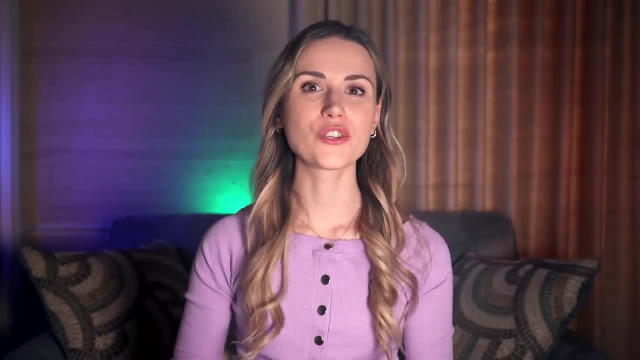 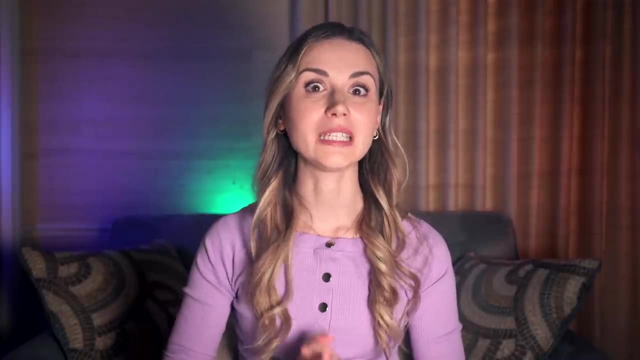 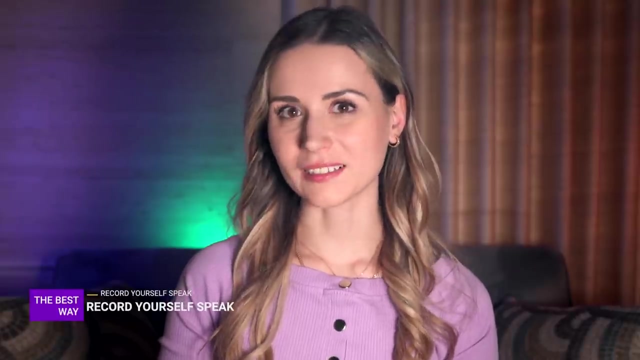 by the way, will come in very handy. Now let's get to the one very thing that you probably won't like, but you will need to do in order to really improve. This way is truly the best and tried and true. You will need to record yourself. speak Nowadays. 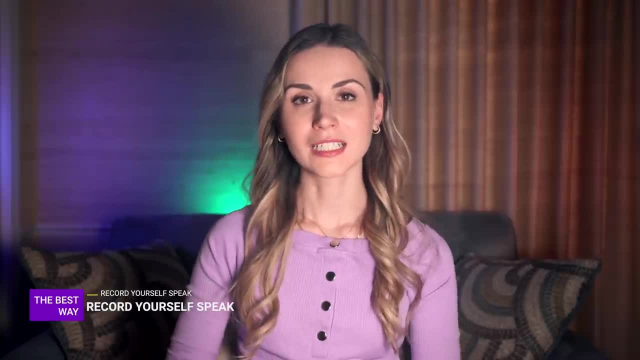 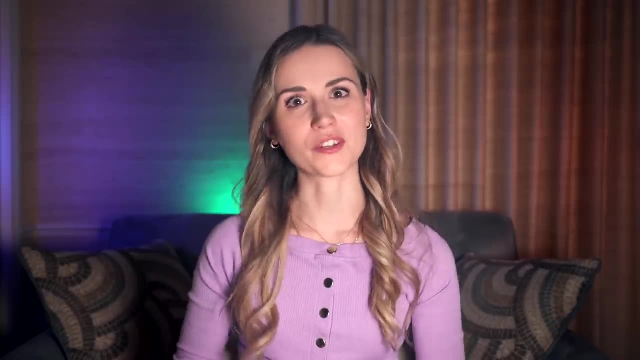 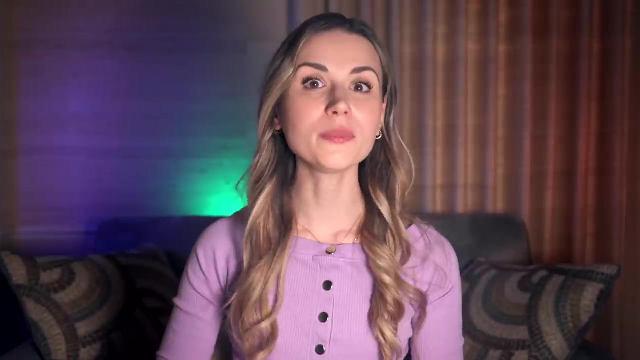 we all have phones with cameras, so this shouldn't be a problem. I know, I know Awkward, awkward, awkward. You feel awkward recording yourself and speaking to yourself. First of all, nobody has to see those videos. Second, you'll get used to it. But believe me, 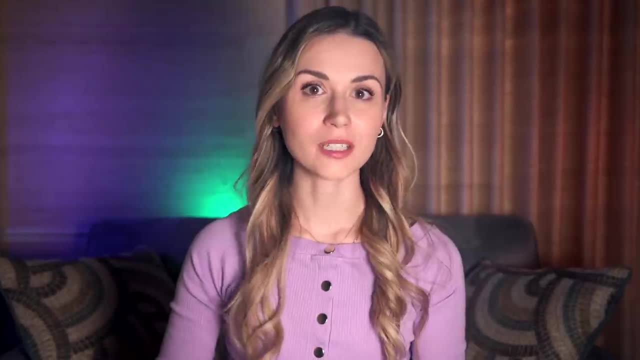 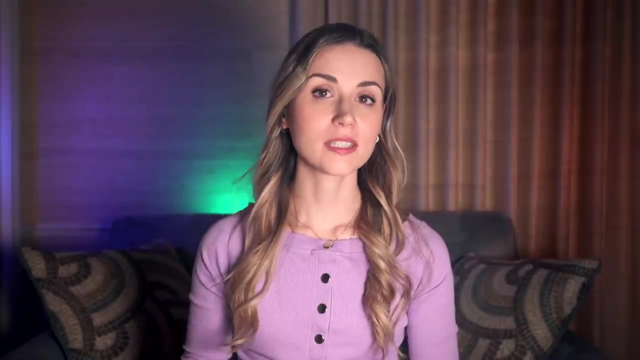 you need this. You need this anyways, but especially because you're working on your own and there's nobody to correct you. When you listen to yourself back, you can catch your mistakes that otherwise you wouldn't even notice you make, whether they are pronunciation or 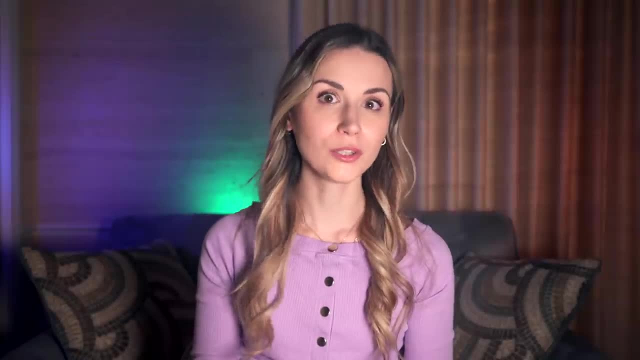 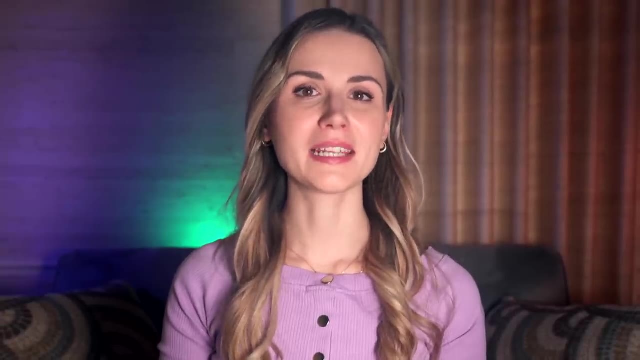 grammar mistakes and you can correct them. I'm telling you this from my own experience making YouTube videos. You won't believe how many takes I needed to take at the beginning to say something right. I could completely butcher a word or the whole sentences. 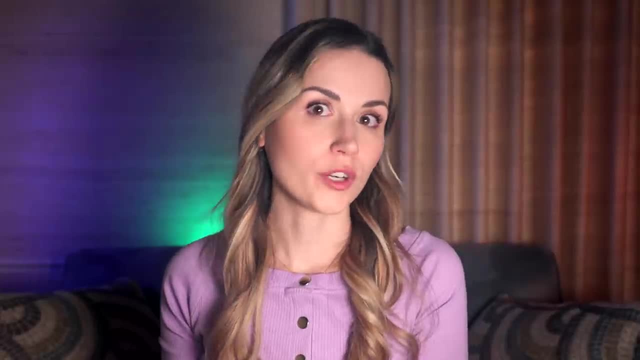 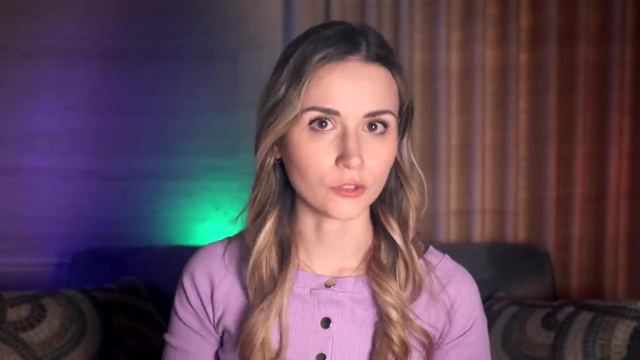 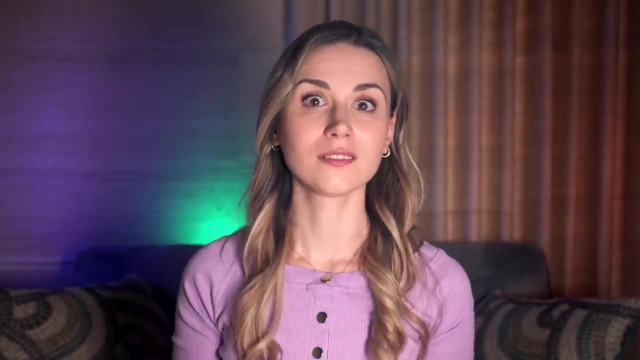 or for whatever reason, I could drop some words from a sentence or my intonation was totally off and consequently the message wasn't properly delivered. But at the moment of speaking I didn't realize that. I thought that everything sounded pretty good. 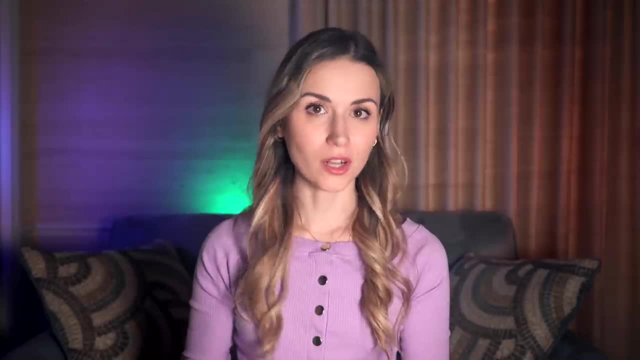 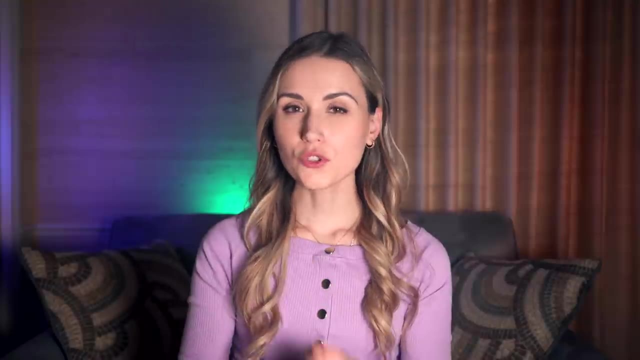 But when you listen to yourself back, you can catch all of that, analyze and correct. And the more you do this, the less you eventually need to do this If you don't know what to talk about or find it difficult to structure your thoughts. 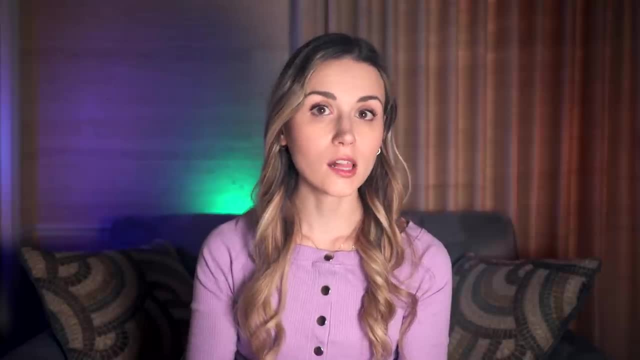 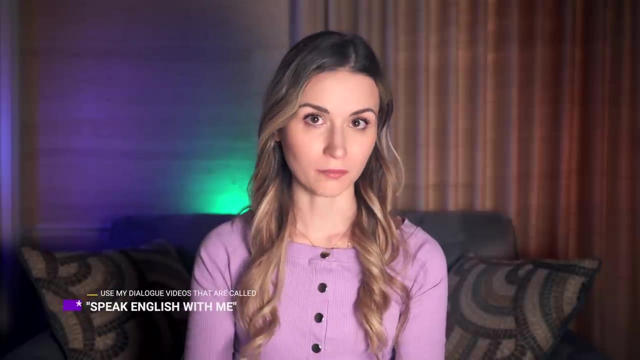 you can start with dialogues. You can come up with them by yourself or find them online, Or, again, you can use my dialogue videos that are called: Speak English With Me. I'll link the playlist with all of those videos in the description. 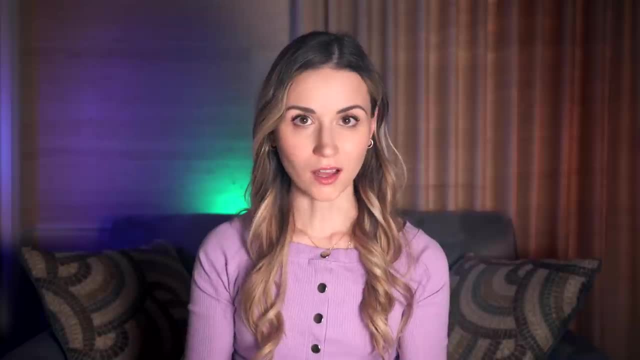 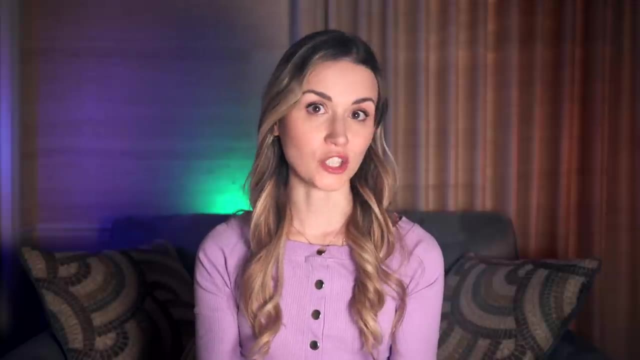 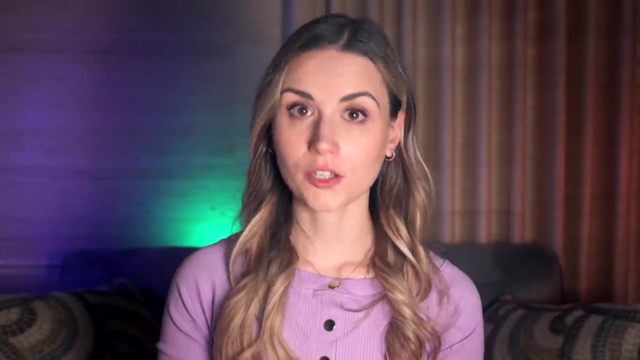 So you can use those already put together dialogues. you can record yourself reproducing the full dialogue, or you can simply answer me, just like the video suggests. Moreover, this way, you will have something to compare your speech to. Another great way to improve your speaking by yourself is to use the app. 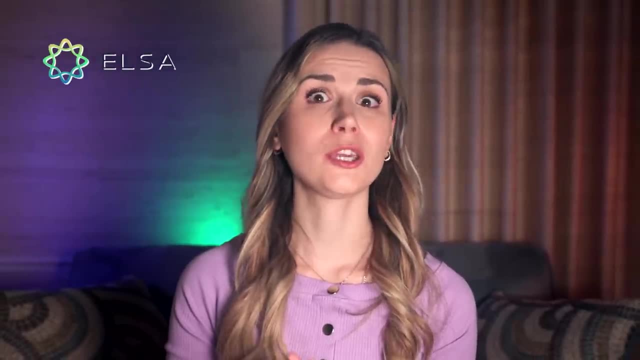 Elsa Speak. They are sponsoring today's video and they couldn't be more appropriate for the topic of today's video. So if you want to learn more about the topic of today's video, click on the link in the description. Elsa Speak helps you improve your speaking and pronunciation in. 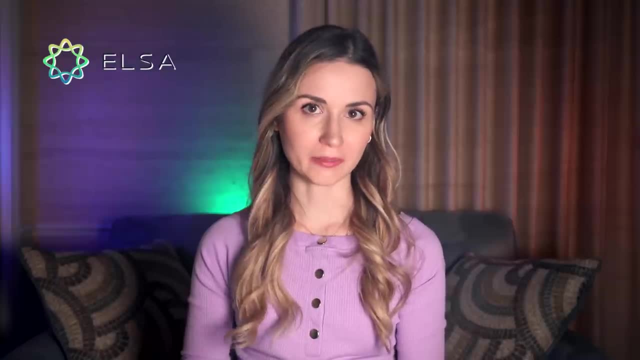 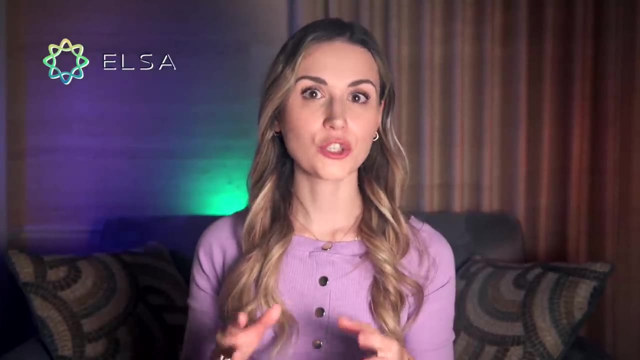 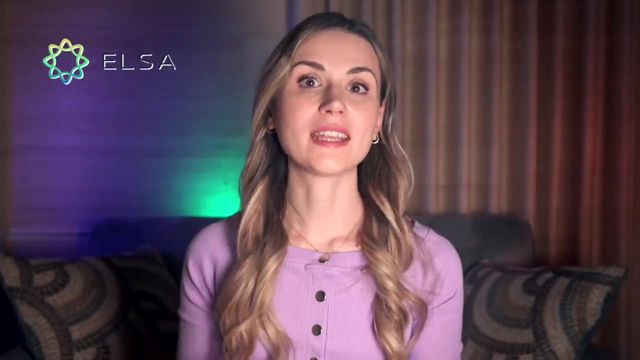 English exactly by means of recording yourself speaking. You can work on individual sounds, separate words and full sentences, And the most awesome and useful part is that the app gives you feedback on your pronunciation with an explanation of what exactly you need to work on, so you don't. 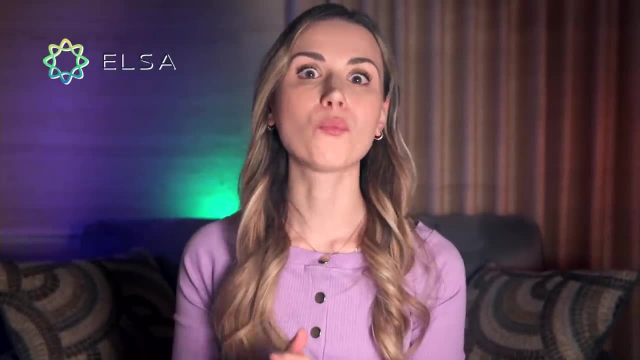 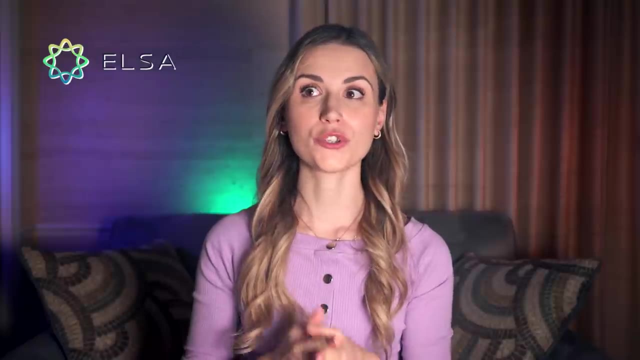 even have to analyze your speech yourself, And there's a lot more cool features. I think that signing up for Elsa Speak can be a wonderful New Year's gift to yourself or to your friend or a family member, especially signing up for their premium membership, you know, to kickstart the 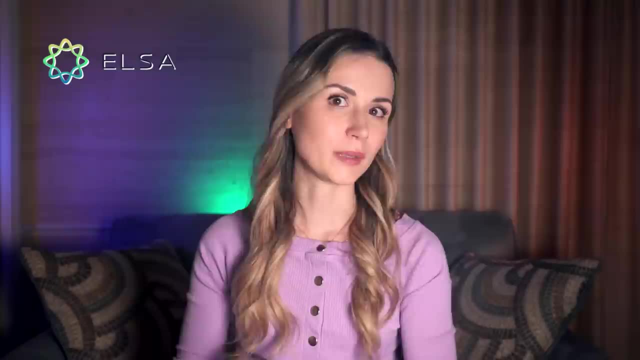 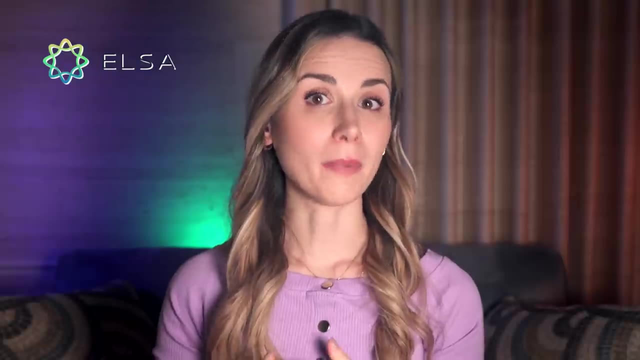 upcoming year by taking a step towards achieving your speaking goals, Which, by the way, is something that I'm planning on doing. I will purchase the Premium Lifetime Membership for my mom- She's really struggling to find a way to practice her English and her speaking- and Elsa 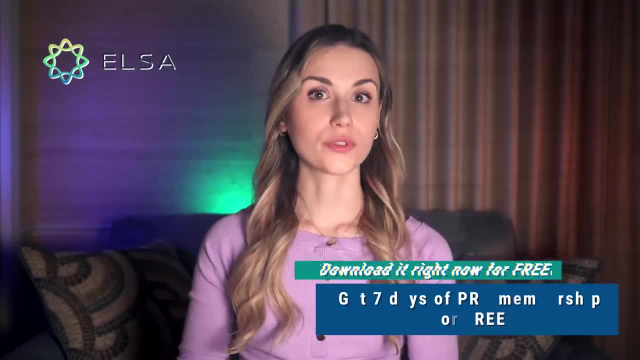 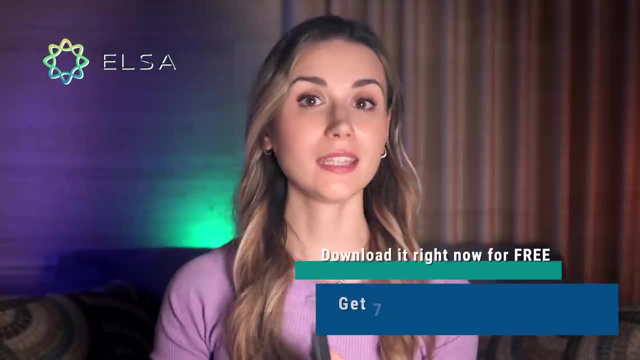 Speak will be perfect for that. So if you want to learn more about the app, click on the link in the description And you can download it right now for free and get 7 days of pro membership for free. The link is in the description and in the pinned comment, And now I'll show you how it works. 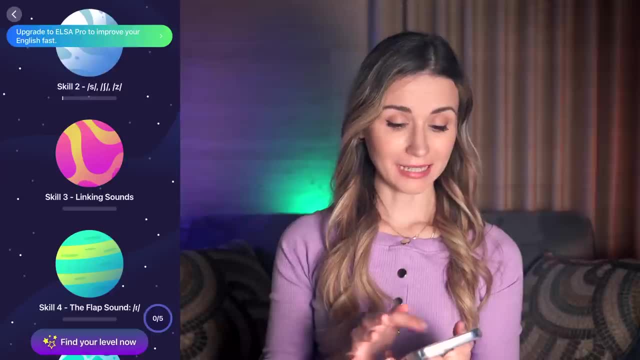 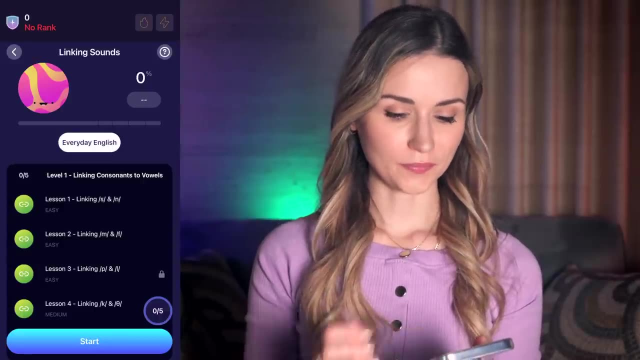 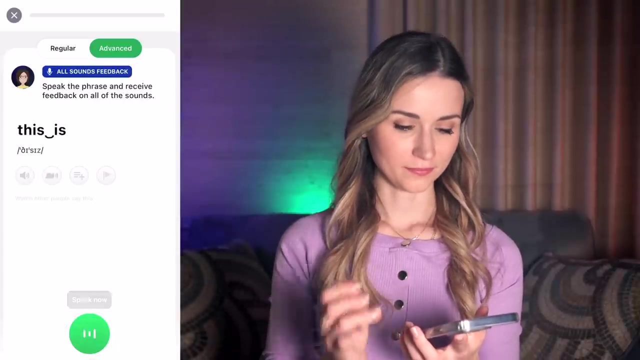 So when you're choosing what you want to work on- let's say, linking sounds- first you get to listen to how the words need to be pronounced And then you'll practice saying them and you'll get feedback on how you did. And then you will look at the words and you'll get feedback on how you did. 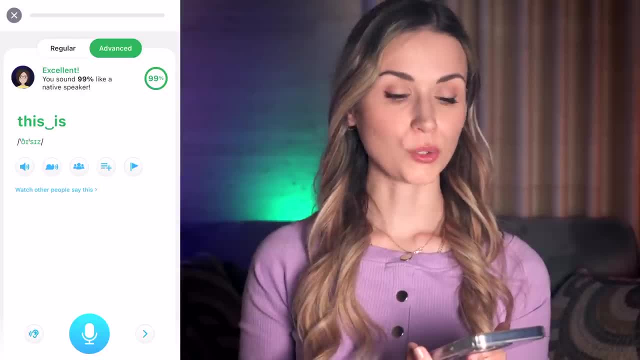 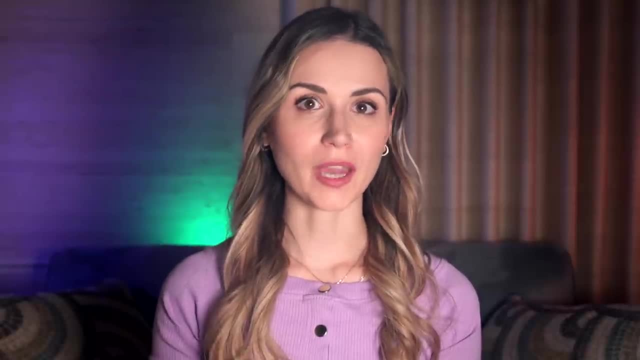 and you'll see how you did. And if you did make some mistakes, you can click on the words and you can see them. And, of course, you can practice as much as you need to master that particular word or sound. And of course, as usual, I have an exclusive discount for you guys to get 85% off of. 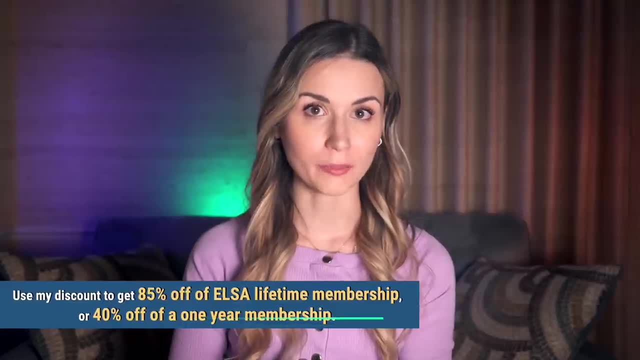 Elsa Lifetime Membership and 40% off of a one-year membership. All you need to do is just click the link down below in the description and it will take you to the link below and you will get a discount. So let's get started.